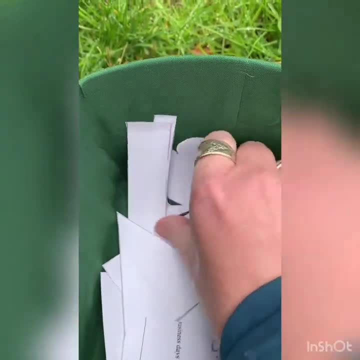 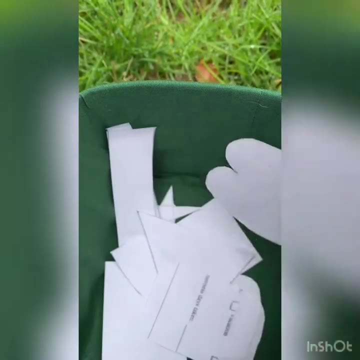 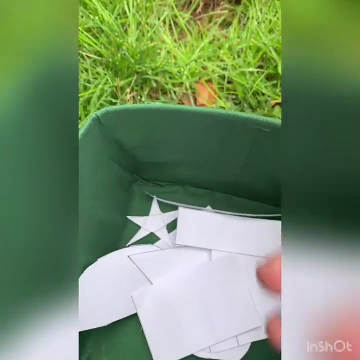 that's a fun one. there's a little rounded rectangle. I tried to cut out a heart. that's scrap paper. yes, it is alright, recycle. so different hearts and different kinds of rectangles as well: fat ones, skinny ones, all different sizes and lengths. so I just came out to my backyard and I looked for some of these. 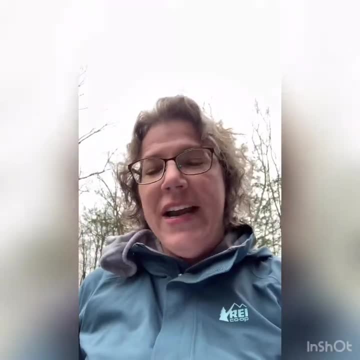 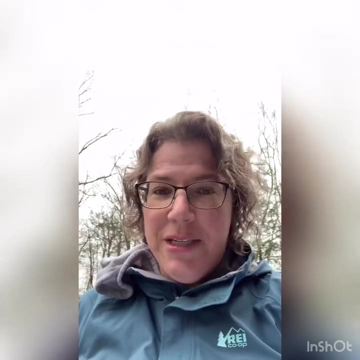 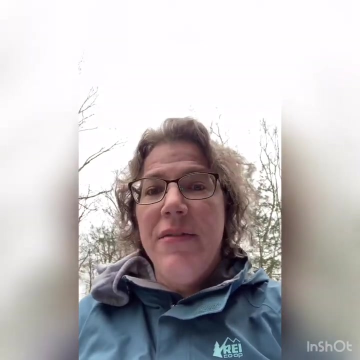 shapes. all right, so those are the different shapes. I just spent a little bit of time going around my yard looking for all those different shapes in nature, and it can become a scavenger hunt- a backyard scavenger hunt- and I didn't pick anything. I found things on the ground, for sure, but I also left the 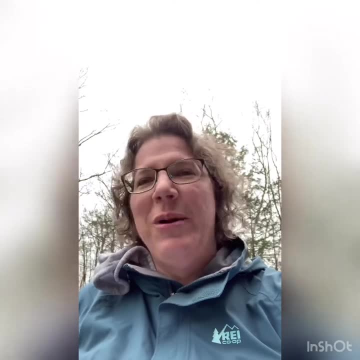 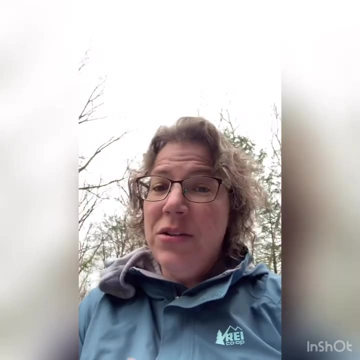 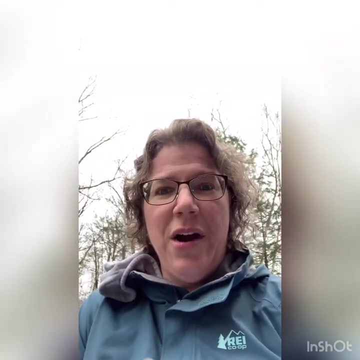 leaves and things of the growing plants, because it is spring and there's actually things coming up now. I left them intact, but what I did was I incorporate art in this. so not only is this a STEM activity- science, technology, engineering and math- it's a STEAM one where you include art, science, technology. 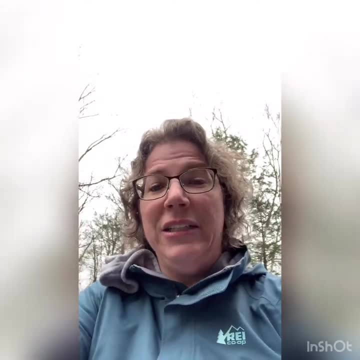 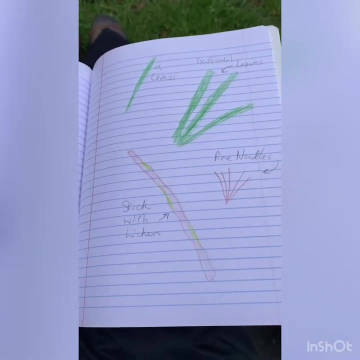 engineering, art and math. so let me show you what I did in my little nature journal. alright, so I just had a composition notebook hanging around my house, so I came out here and spent a little time doing some drawing. so on this page you can see my composition notebook. and I'm going to go ahead and 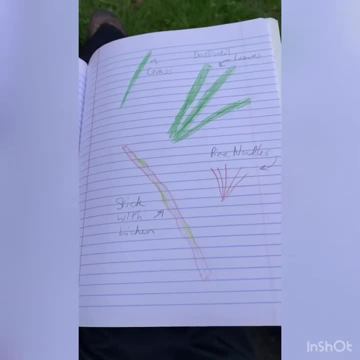 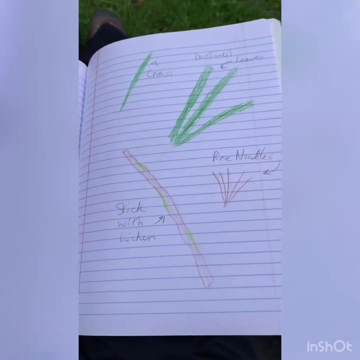 see that I have all of my long skinny rectangles, so there are some daffodil leaves, I found some pine needles on the ground, I found a stick with some lichen and I found some grass. on the other page, I found all kinds of ovals and and. 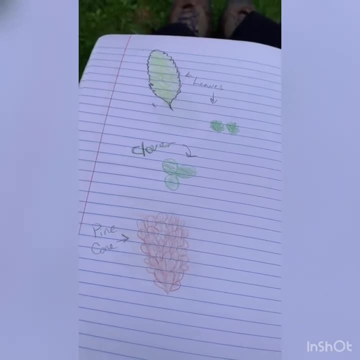 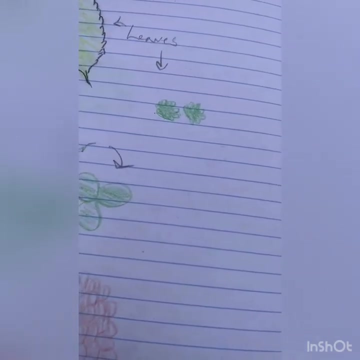 different kinds of circles. so I found a leaf that was oval shaped and it had some teeth on it, so I did that. there are some smaller leaves there that I tried to try to get in there, and those ones also had some teeth on it. I found some clover and I found a pinecone that was 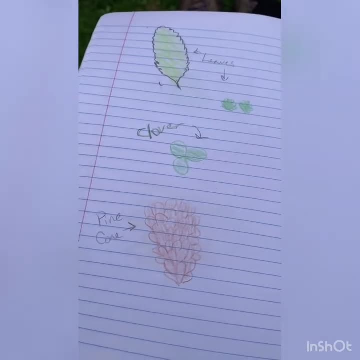 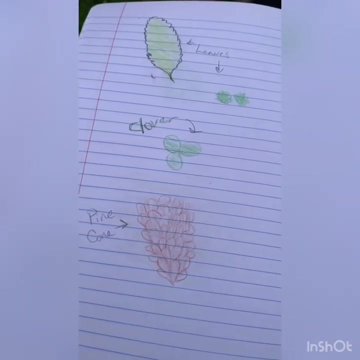 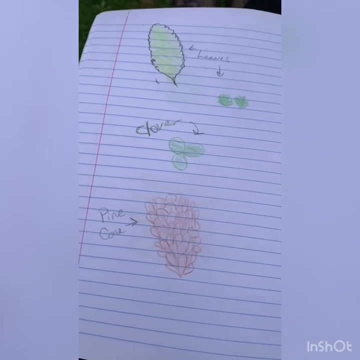 kind of oval shape as well. you can see that I labeled them, so, again, this would be a nice one for the older kids to do the sketching and the labeling. I could have gone into more detail to. these little leaves right here were actually thick and waxy, so I could have given some great descriptive words to these as.